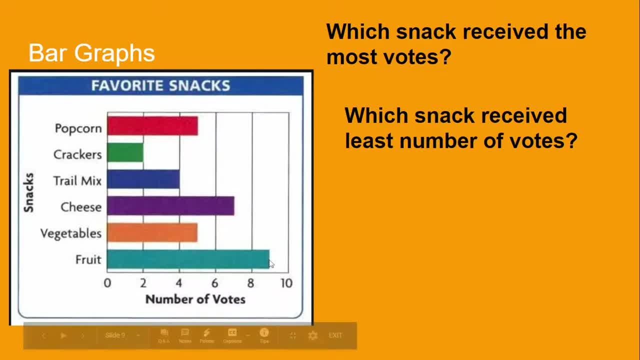 the bar that's the longest to find which one shows the most. So if I look at my bars and I compare them, the longest bar is my blue one, right here. So which snack goes with the blue bar? That would be fruit. So fruit received the most votes. 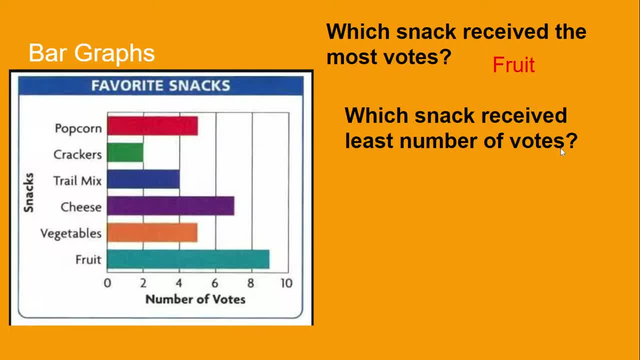 Which snack received the least number of votes. So to find the least number, I'm going to look for the bar that's the shortest. So I'm going to compare. Since this one was the longest, I'm looking for one that's a lot smaller. If I look at each bar, the one that's the shortest. 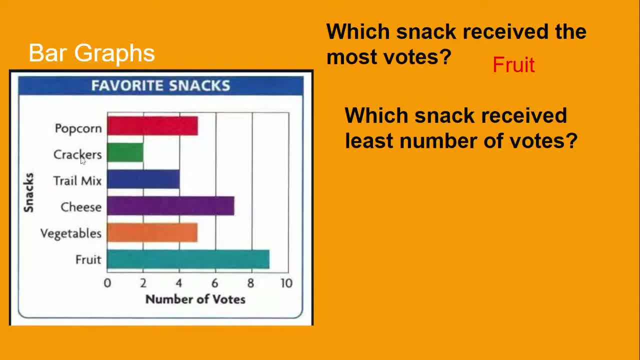 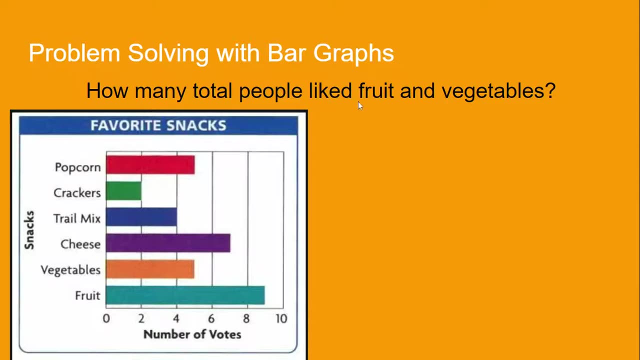 is my green bar. That goes with crackers, So the snack that's the shortest is my green bar. The snack that received the least number of votes would be the crackers. It only received two votes. Let's try solving another problem: How many total people liked fruit and vegetables? 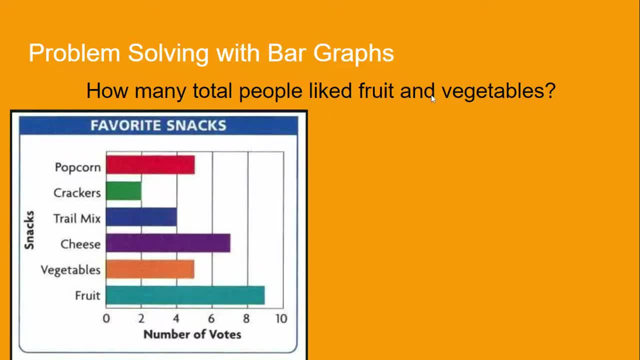 So I see words like total and fruit and vegetables. So that tells me I need to combine these two categories: fruit and vegetables. I'm going to come over to my bar graph and find fruit and vegetables. I'm going to come over to my bar graph and find fruit and vegetables. 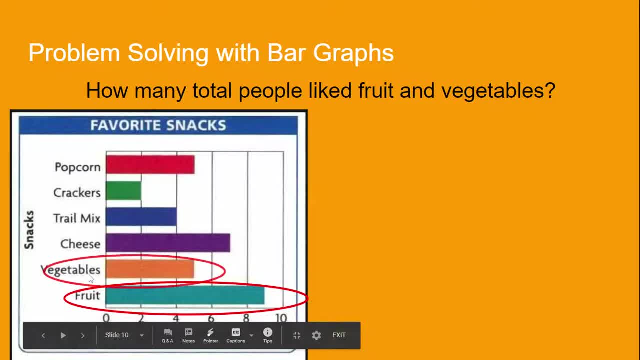 I'm going to come over to my bar graph and find fruit and vegetables. Fruit got nine votes. Remember, if a bar falls between two numbers, it's going to be the number in the middle. So the number between eight and ten is nine. Vegetables received five votes. It falls right. 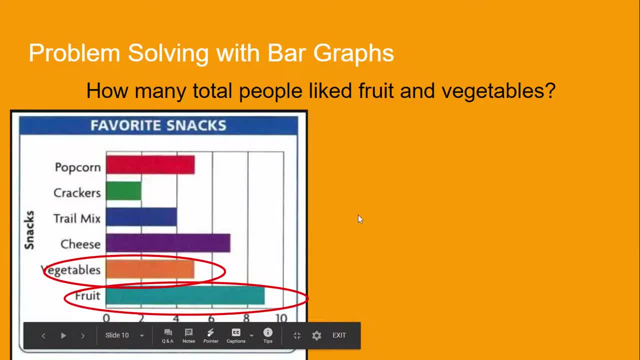 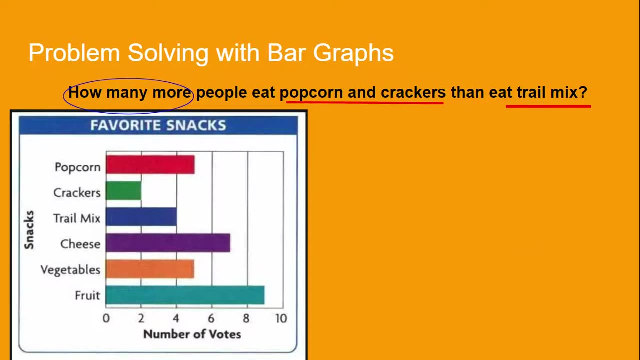 in between four and six, So I need to add nine and five. So nine plus five equals 14.. So I know 14 people liked fruit and vegetables. Let's try another one: How many more people eat popcorn and crackers than eat trail mix? I see those words. how many more? And I want to know how many people. 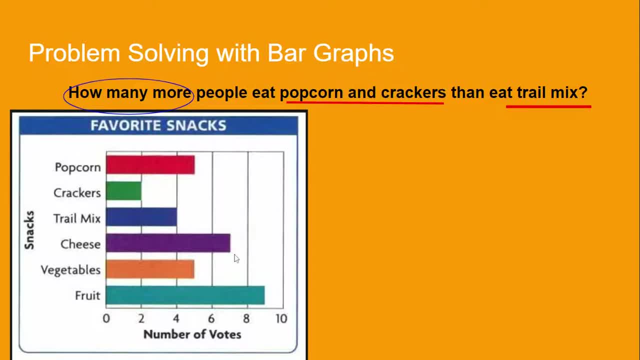 eat popcorn and crackers than eat trail mix. So let's start with our popcorn. That's five votes And our crackers. That received two votes. So I need to add those two numbers And that tells us to put those numbers together. Five plus two equals seven, So I know seven people.